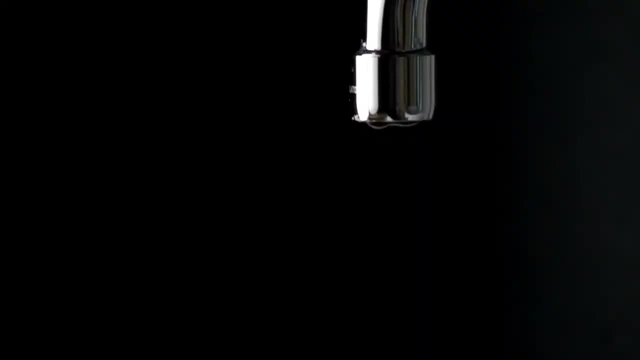 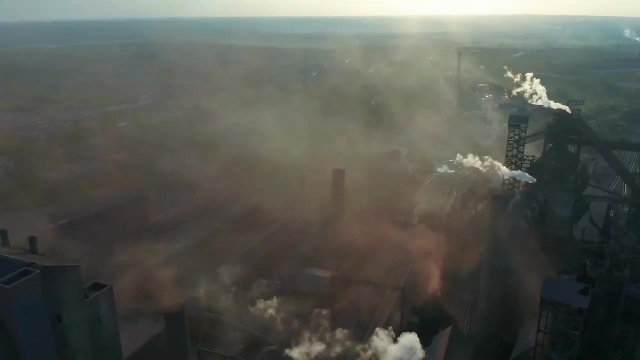 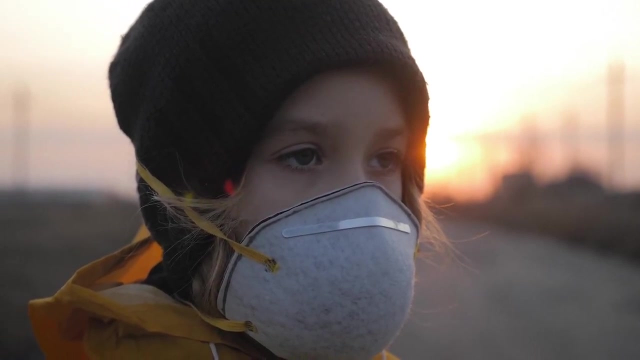 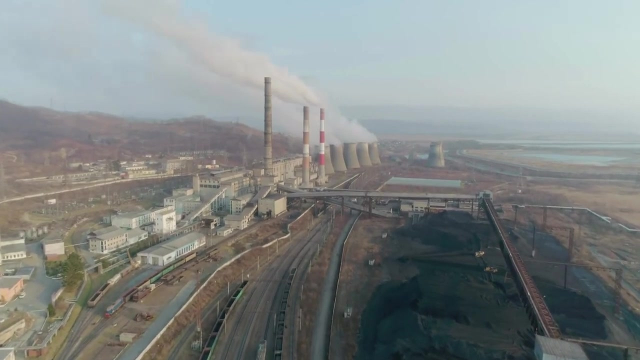 food security, water supplies, infrastructure and economic activity Sounds pretty gloomy right, And it really is The good news, though. there's plenty of things we can do as individuals, communities, countries and globally to slow human-induced climate change and help save our precious planet. 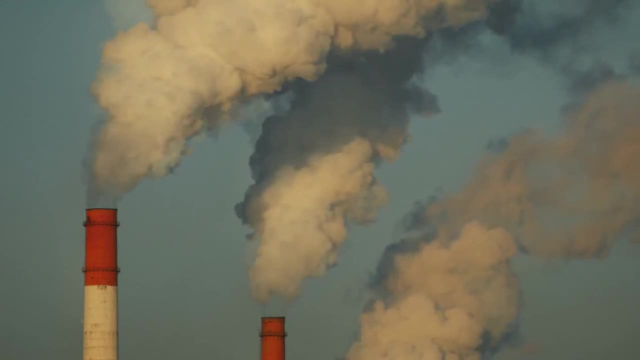 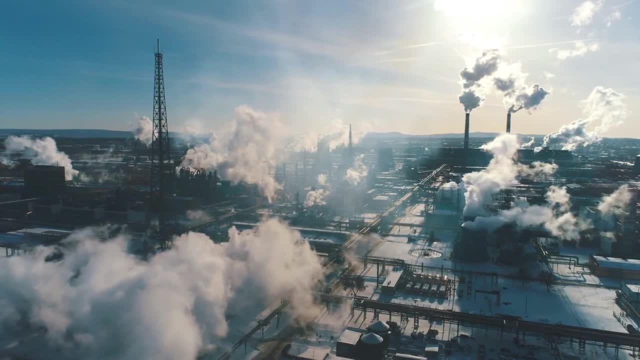 is a major contributor to the global climate crisis. The global climate crisis is a major contributor to the global climate crisis. Elements of climate change can be clarified quickly, but it's like having been foxed in bed for several seconds. but a잖아요ny. 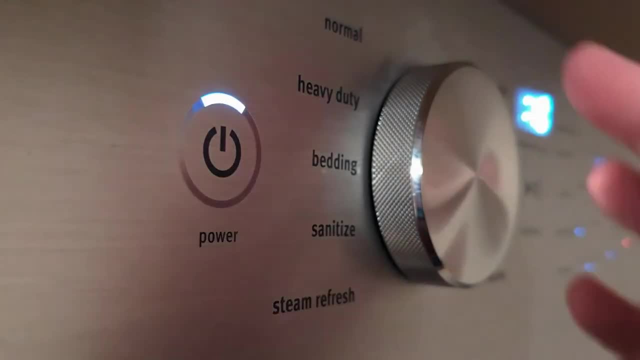 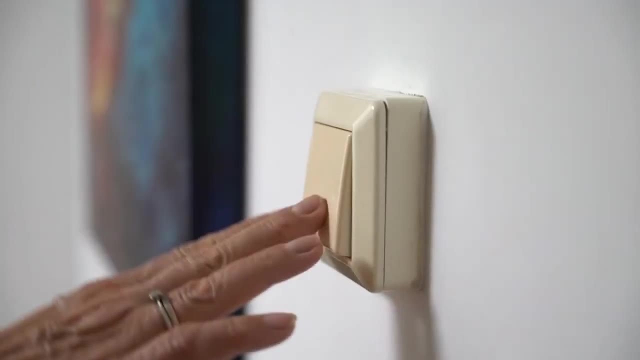 What it takes is the human right to act and forthe 말� of the world we all know has consequences for planet基 28.. Earth 19 and energy generation can be hampered on the way shown in the parks waterاحlogs. 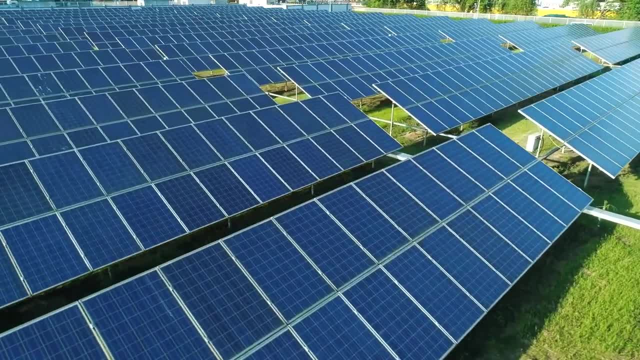 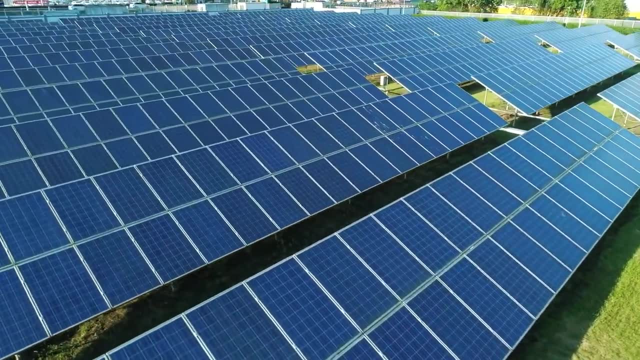 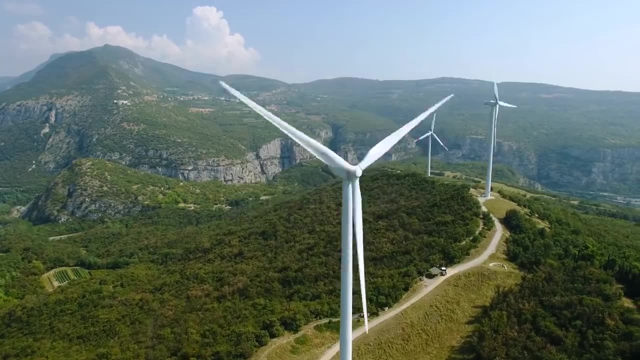 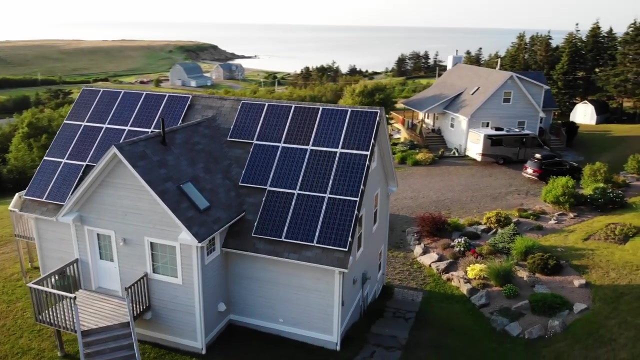 assuming a backup climate, which energy at an trênoloaseote? We can also encourage local governments to adopt renewable energy sources such as solar, ER, hydro and wind power. you can also take matters into your own hands by installing solar panels on the roof of your house or school. this way, you'll 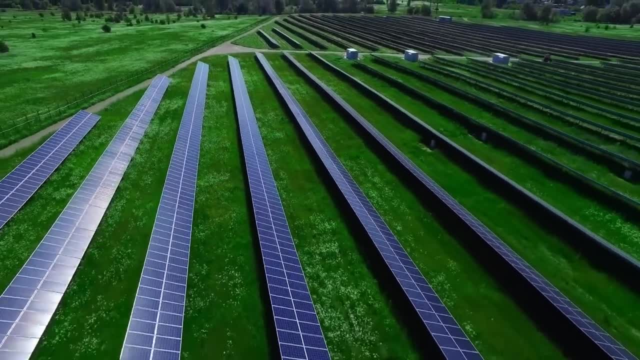 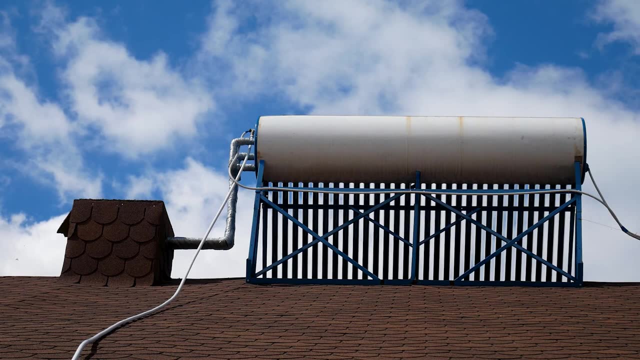 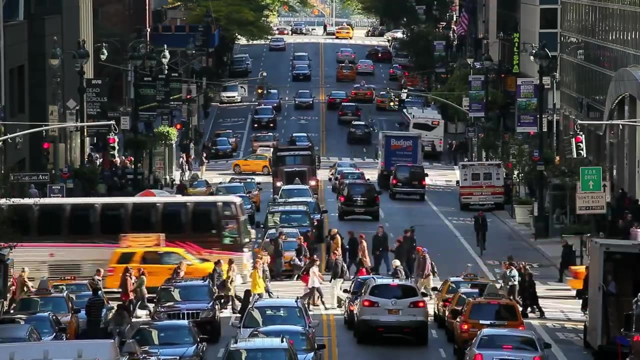 meet all or most of your electricity requirements using the clean renewable energy from the Sun. you could also use a solar water heater to provide your household with warm water for bathing and washing. fossil fuels are also burned to power the vehicles we use, including motorcycles, cars, buses and trucks. 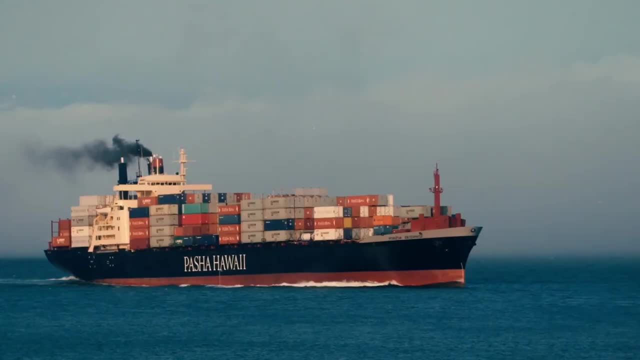 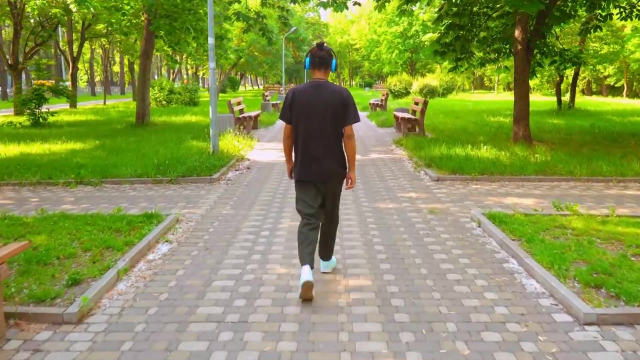 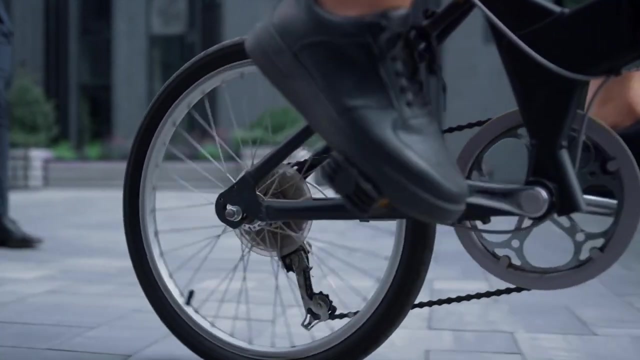 airplanes and ships to reduce greenhouse gas emissions from vehicles. we can simply use them less often. if your school or local shops are nearby, try walking or walking on the street, and you'll be able to use your household or riding a bike. in recent years, the use of electric vehicles are becoming more 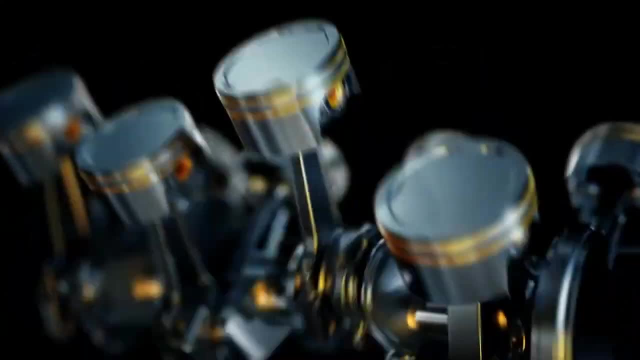 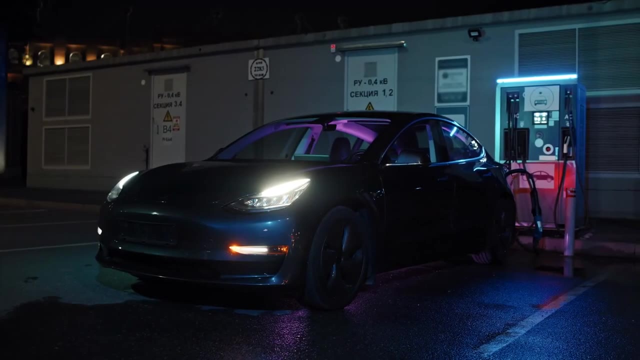 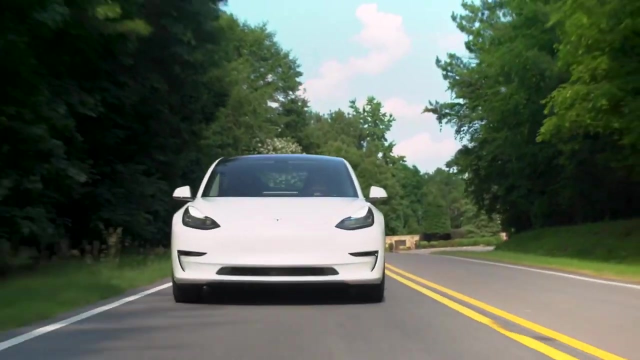 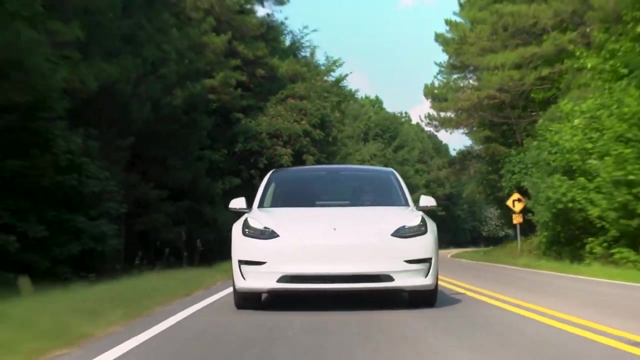 and more popular. rather than using a combustion engine that burns petrol, diesel or gas, an electric vehicle runs purely on electricity and has the same performance as a vehicle with combustion engine, sometimes even better. switching to electric vehicles will also drastically reduce hazardous air pollution in our cities. trees and forests play an important role in reducing greenhouse gases. 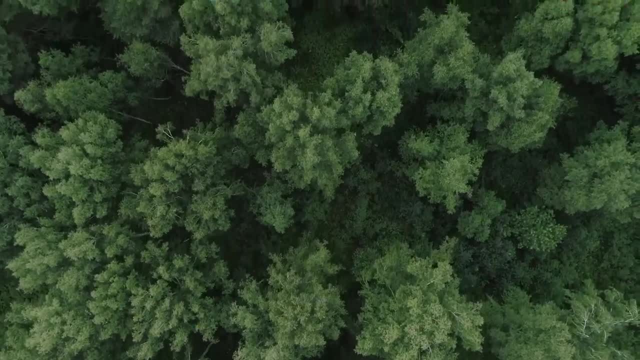 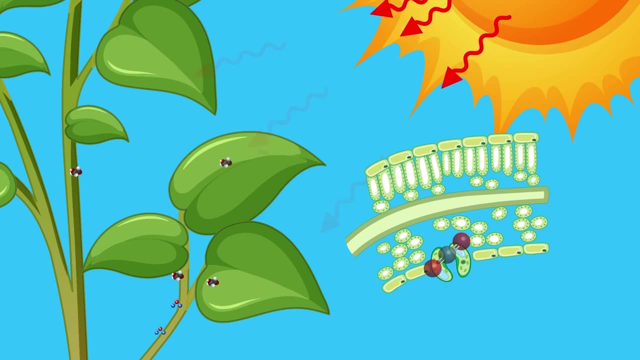 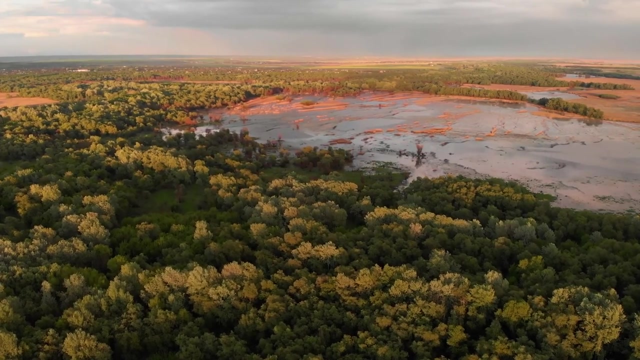 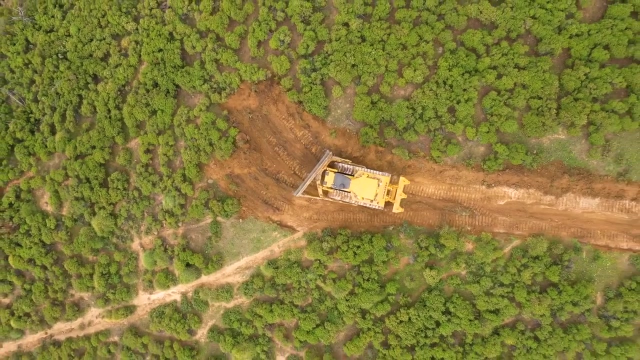 because they act as a carbon sink. when trees and other plants photosynthesized, they absorb carbon dioxide from the atmosphere and store it in their tissues. in this way, they helped to offset the greenhouse gas emissions that come from human activities. when humans come along and clear forest for land use, a process called deforestation, we prevent this absorption. 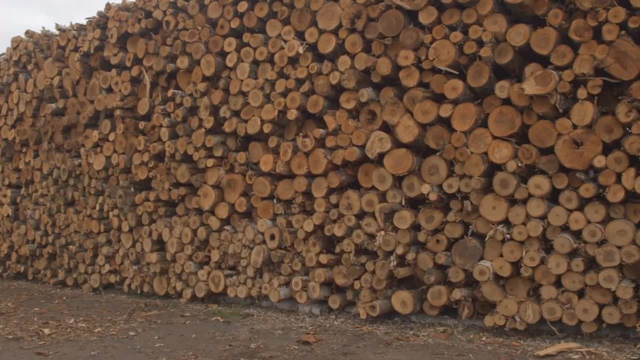 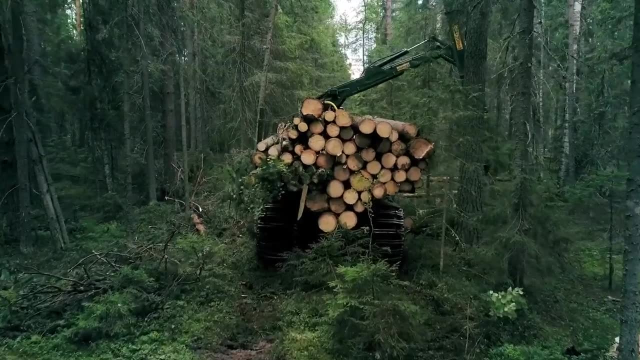 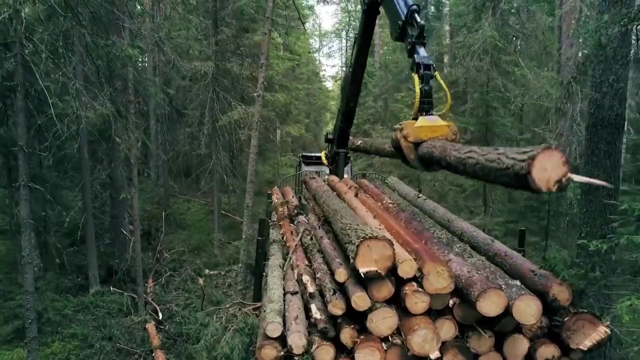 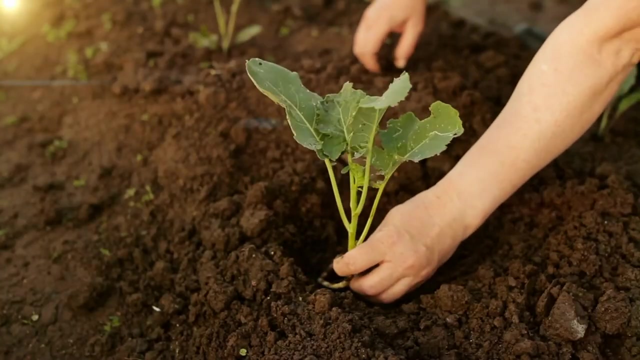 of carbon dioxide from the atmosphere, again contributing to increased greenhouse gases in the atmosphere. We can encourage governments to stop deforestation and only use timber from sustainable forests whereby the trees grow back at the same rate they are being used. Planting trees and plants is another way you can be actively involved in reducing greenhouse. 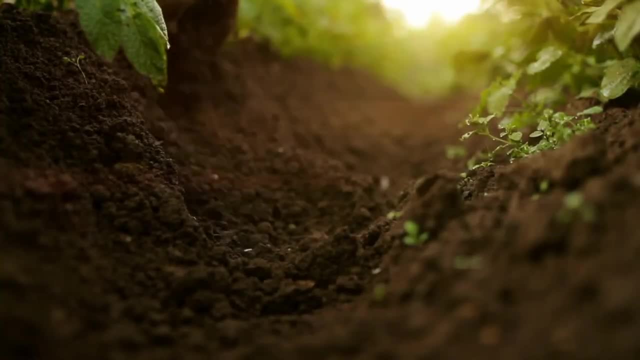 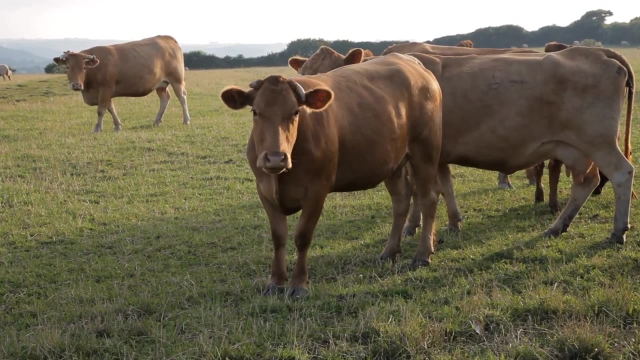 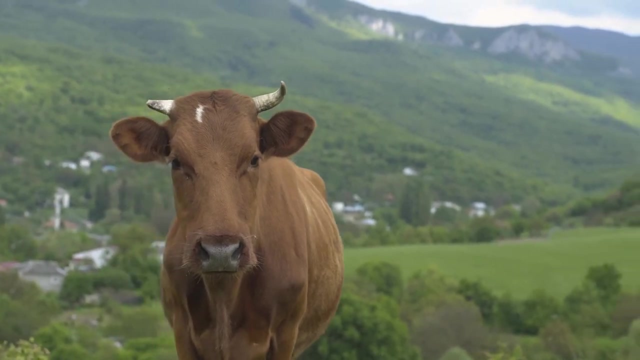 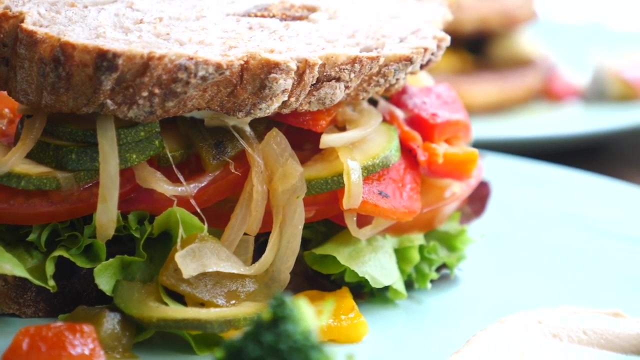 gases. Check if any tree planting activities are taking place in your community. You may recall that cows are an unlikely contributor to increased greenhouse gases in our atmosphere. Release the greenhouse gas methane. To reduce methane emissions from cows, we can simply choose to eat less meat and focus. 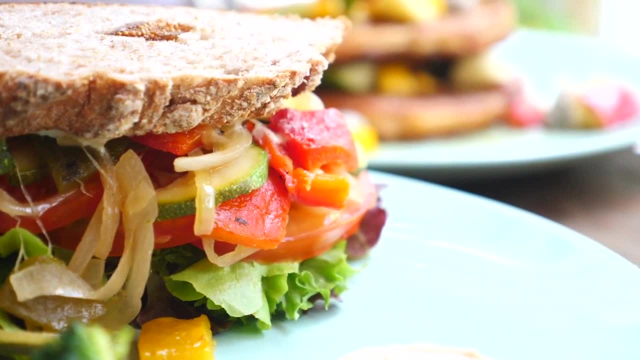 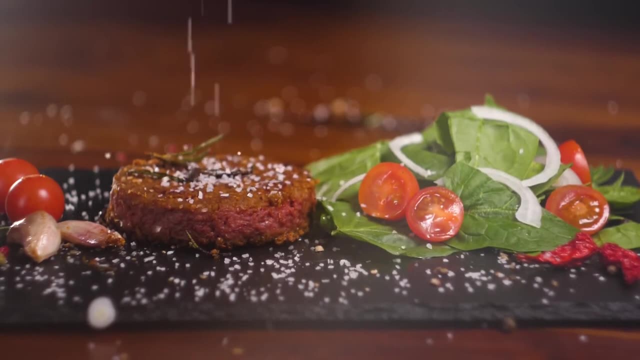 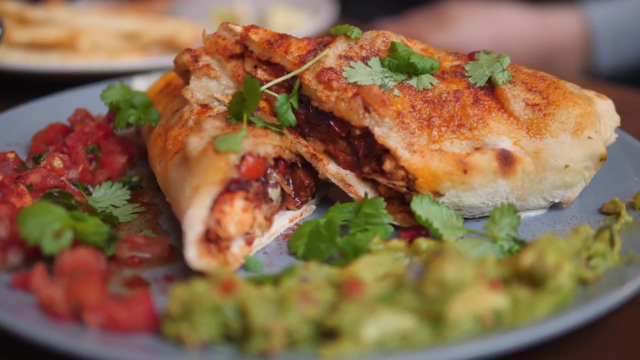 on a more plant-based diet. In recent years, scientists and food nutritionists have developed traditional meat products like minced beef, burgers and sausages that are made entirely of plants. Many meat lovers cannot tell the difference between these plant-based protein foods and